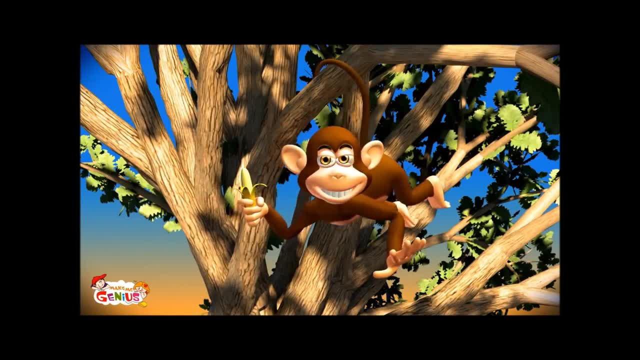 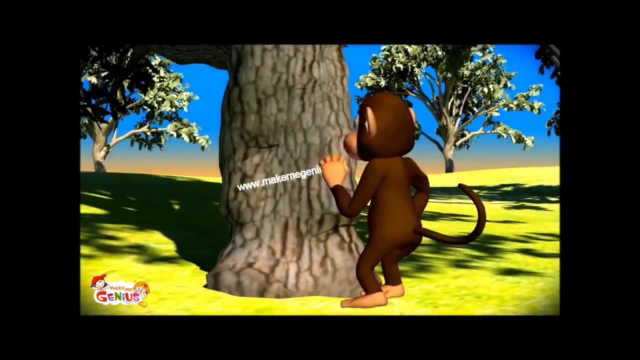 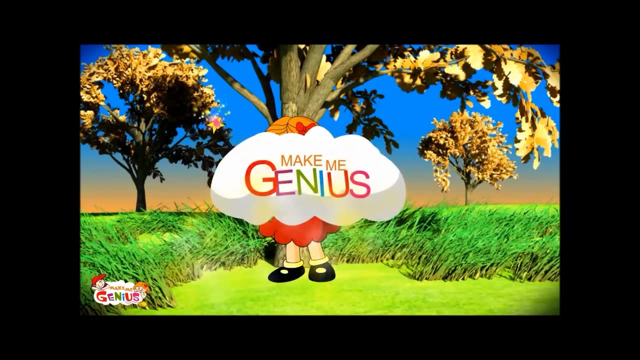 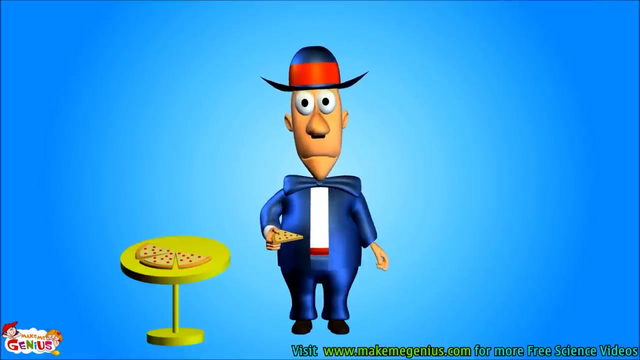 This video is from wwwmakemegeniuscom. If you want to see more science videos, go to wwwmakemegeniuscom. Yeah, it is free. Hey, lucky man, Can you give a bite to me If I tell you something about pizza and food. would you give a piece? 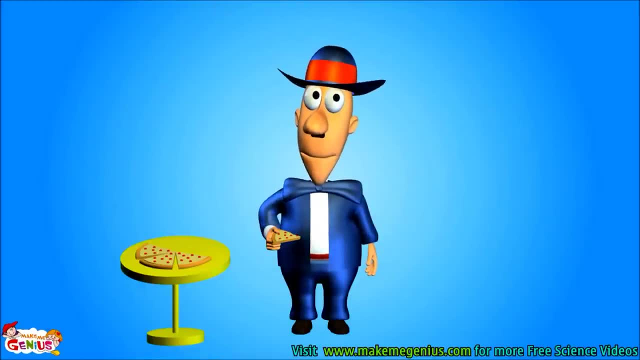 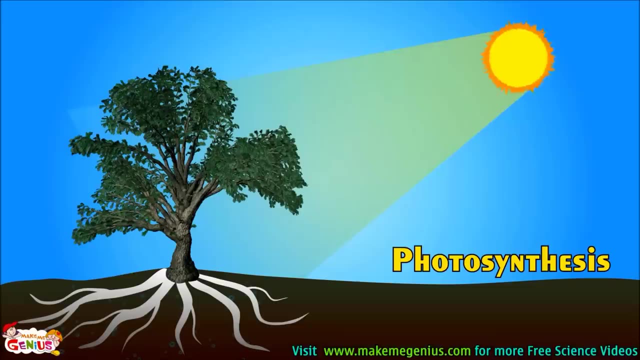 Okay, Tell me, do you know where all food comes from? Wow, you are right. We humans get all our food from animals and plants. Let me tell you more about food. Plants are only living species who make their own food. They use sunlight, carbon dioxide from air and water from soil to make their food. 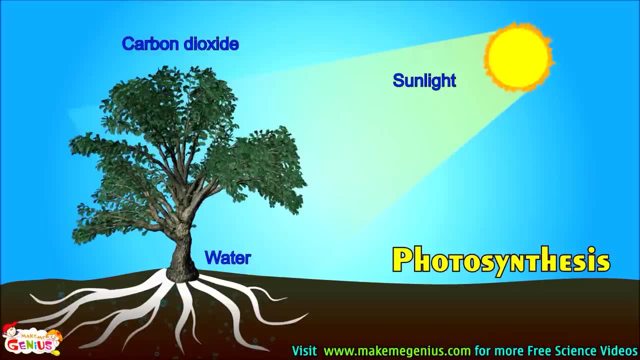 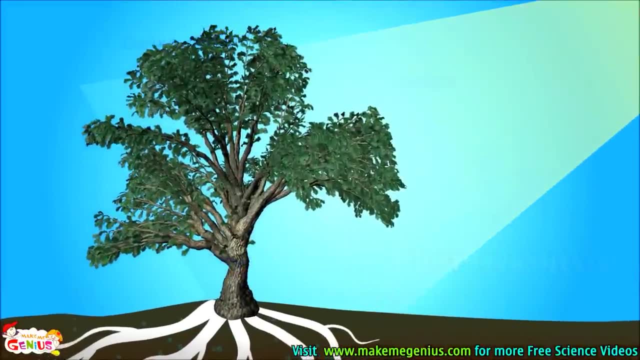 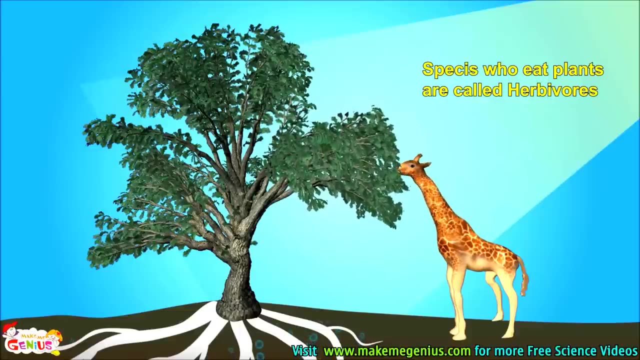 This process is called photosynthesis. So now you know, plants make their own food. All other species, like animals and we humans, are dependent on plants. Now see, A giraffe is coming. It is eating. the plant Species who only eat plants are called herbivores. 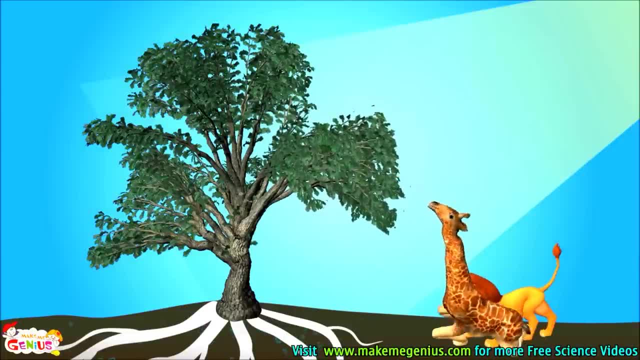 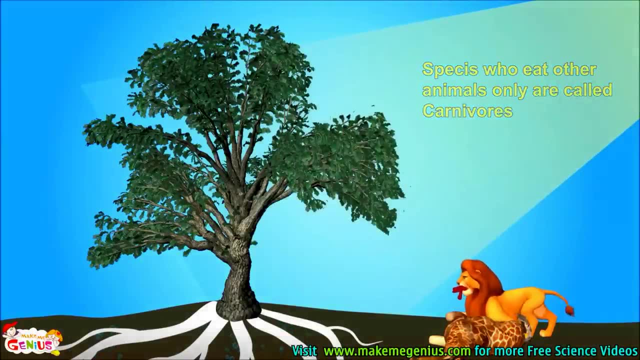 Oh, what is happening? A lion is coming. Oh, it is attacking the giraffe. Oh, it has killed the giraffe and is eating it. Species which eat other animals are called carnivores. So you have seen plants make their own food. 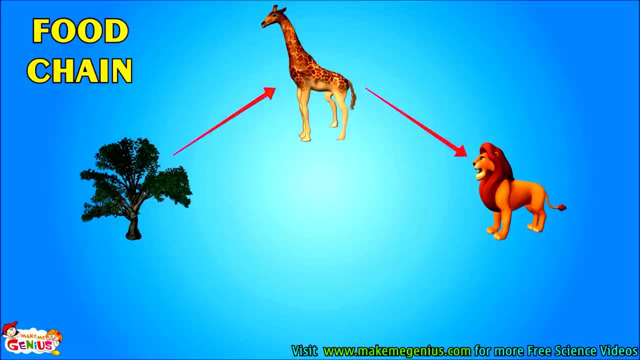 Other animals eat plants and some other animals eat those animals who eat plants. So all are dependent on plants. This is also called food chain. It starts from plants. In food chain, plants are known as producers as they produce food. The species who eat plants are called primary consumers. 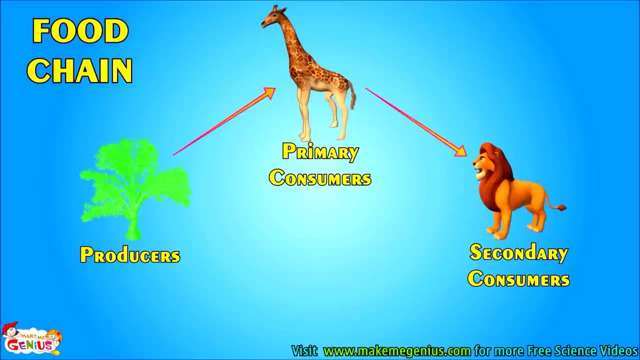 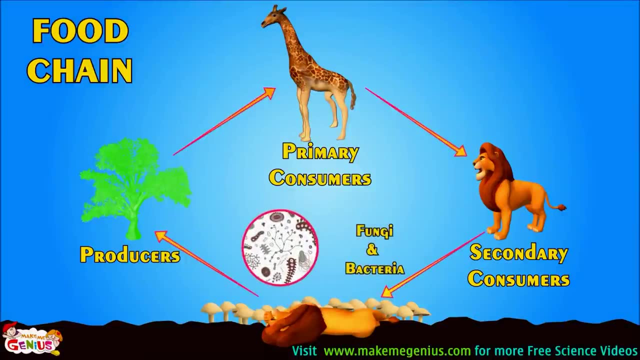 And the species who eat, species dependent on plants, are called secondary consumers. Now there is one more part of this food chain. These are fungi and bacteria in soil. When animals die, these fungi and bacteria in soil decompose their dead bodies. They become nutrients. 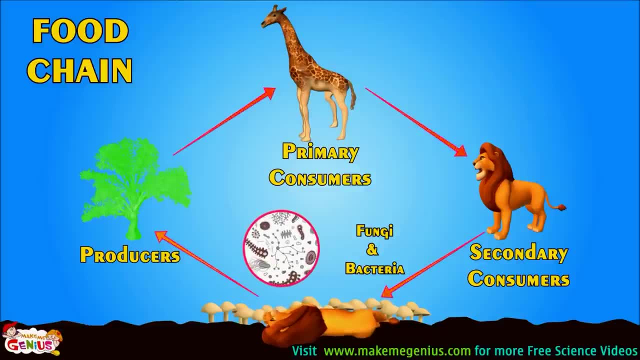 These nutrients again are used by plants to make food. See here: When lion dies, its body is decomposed in soil by bacteria and fungi And it turns into nutrients. Then these are again used by plants. These fungi and bacteria are called decomposers. 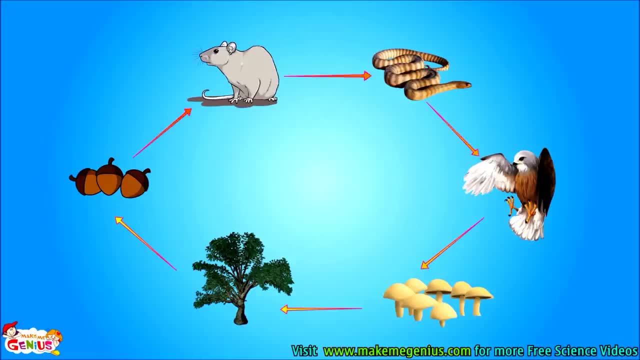 Decomposers are an important part of food chain. Let us see other food chains Here. rat eats acorn's fruit, which comes from plant, And snake eats rats. Eagle eats rat Eagle dies. It gets decomposed And plants use decomposed nutrients to produce fruit. 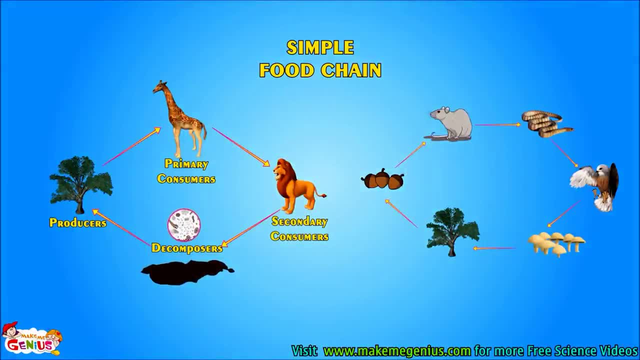 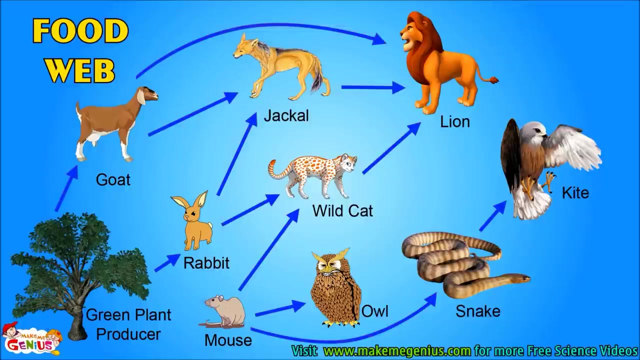 The food chains which we saw, which have one producer, one primary consumer and one secondary consumer, are called simple food chains. Actually, life is not so simple. Look at this picture. This is very complex. Look at the rat. It can be eaten by cat also. 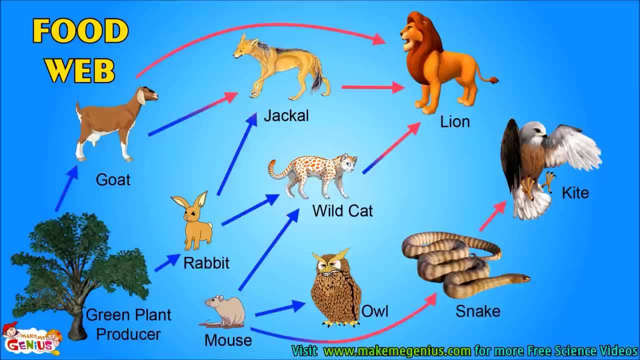 Or it may be eaten by snake Plant can be eaten by goat or by rabbit. These kind of complex food chains are called food web, as they are very interconnected like a spider web. So now you know a lot about food food chain and food web. 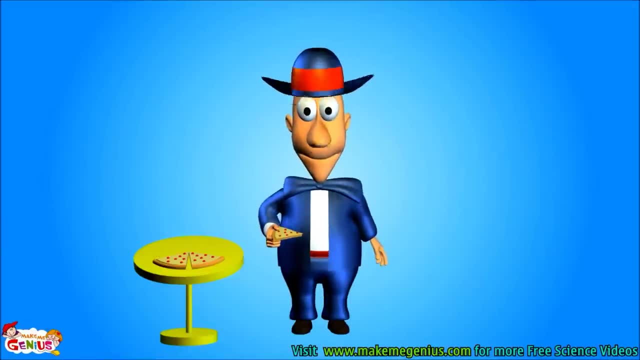 Now. can you give me a piece? Thank you, I was so tired and hungry, I wanted energy to continue. Do you know why we need food? Okay, okay, You know, You know we need food to get energy. Energy is required by living being for growth, also for movement. 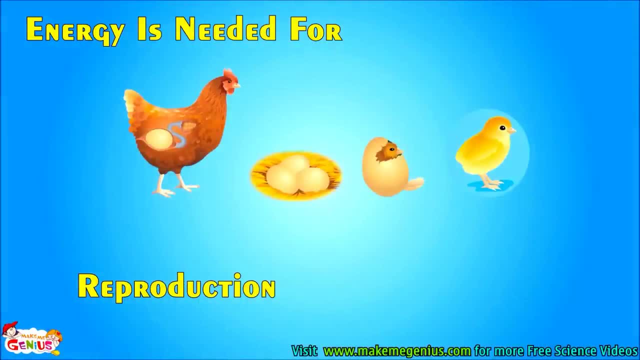 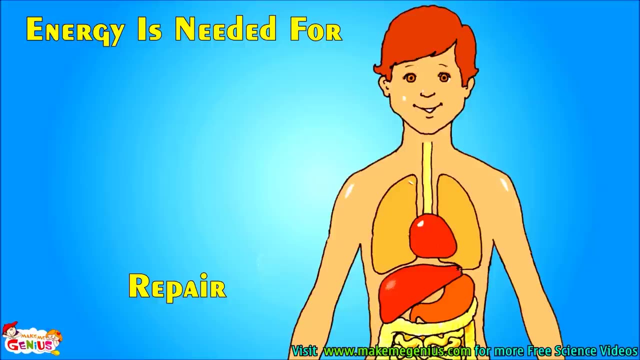 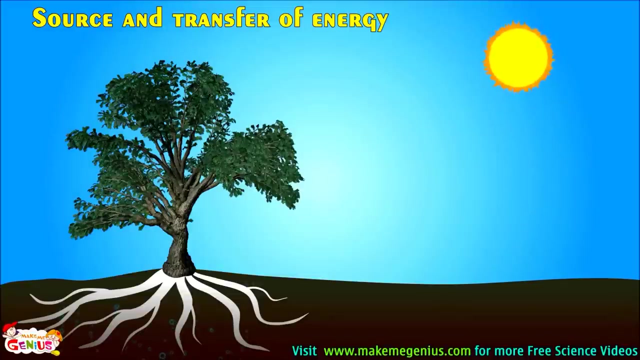 We need energy. Similarly, when species reproduce, they need energy Also, as grow up or grow old, our old tissues get damaged or new cells are produced. This process also needs energy. Now from where this energy come from? Most of the living species use sun's energy. 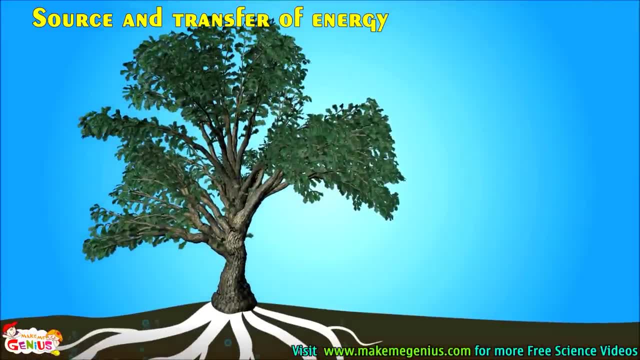 This energy is transferred to body via food they eat. Sun gives light energy which is used by plants to make their food by photosynthesis. These plants are eaten by primary consumers and energy is transferred to them. Now, secondary consumers eat these primary consumers and energy is transferred to them too. 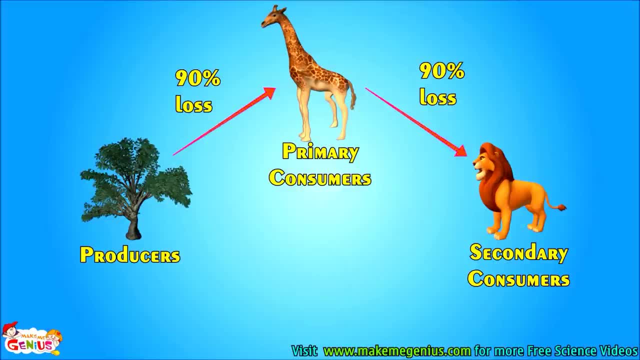 So does giraffe get all the energy from plant? which plant gets from sun? Or does lion gets all energy from giraffe? which giraffe gets from plant? The answer is no. Actually, 90% energy is lost. The answer is no. 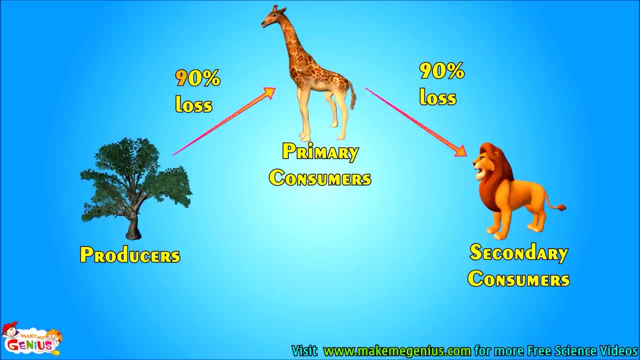 Actually, 90% energy is lost when it passes from one part of chain to other, Like 90% energy is lost when giraffe eats plant. Similarly, 90% energy is lost between lion and giraffe. Look at this pyramid.